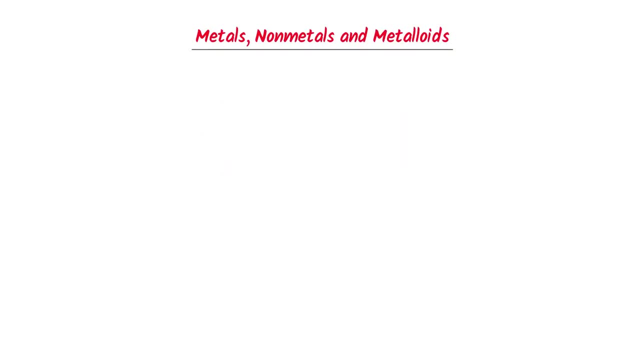 Metals, non-metals and metalloids. We know that there are 118 elements present in the universe. All these elements are classified into metals, metalloids and non-metals. Out of these 118 elements, 92 elements are metals, 6 elements are metalloids and 20 elements are non-metals. 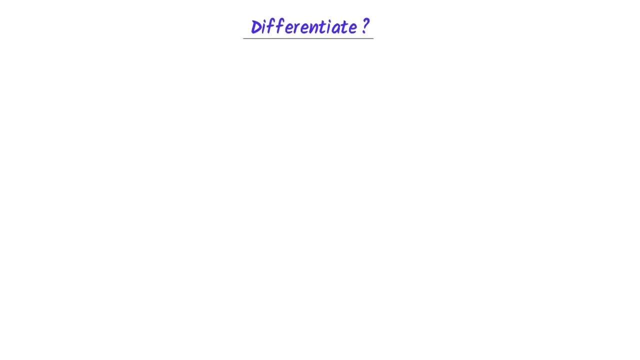 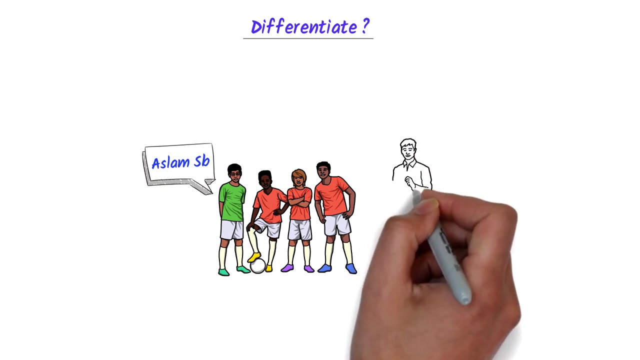 Now, how can we differentiate among metals, non-metals and metalloids and the periodic table? Well, I always teach my personal trick. Consider a football team of your class. Let Aslam Saab is the captain of this team. Now, every year, Bayusar picks Aslam Saab team. 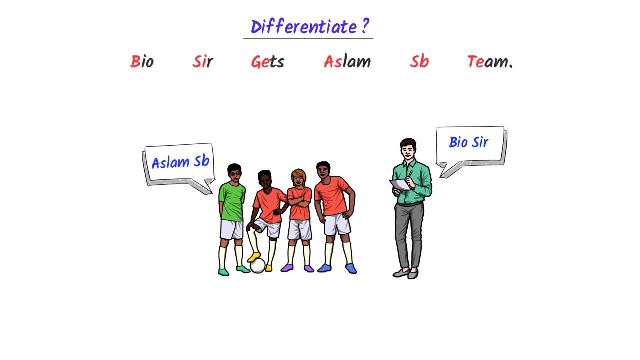 So I say Bayusar gets Aslam Saab team Here. B stands for Boron, Si stands for Silicon, Ge stands for Germanium, As stands for Arsenic. Sb stands for Antimony and Te stands for Tellurium. These are the 6 metalloids in the periodic table. 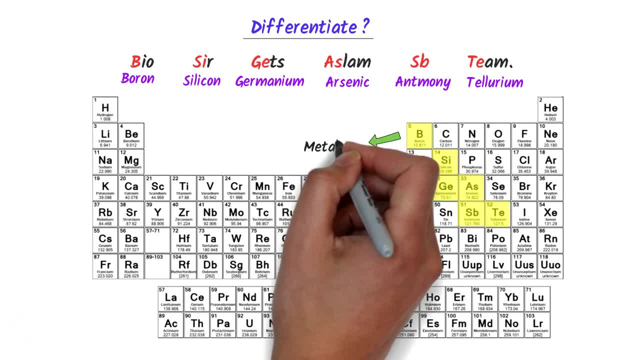 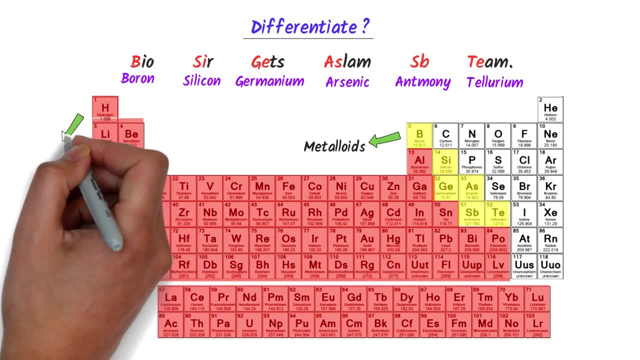 Thus, I highlight all these 6 elements in the periodic table. Now listen carefully. At the left sides of the metalloids, all these elements are metals, While at the right side of the metalloids, all these elements are metals. Now listen carefully At the left sides of the. 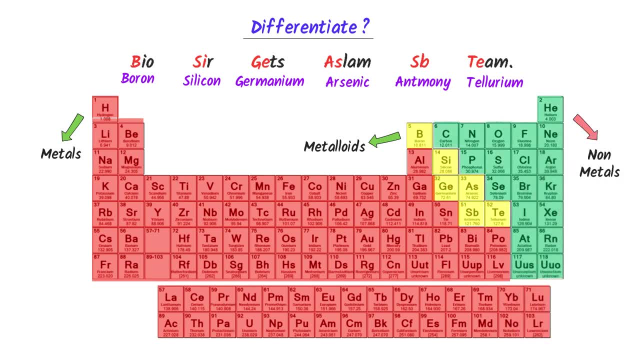 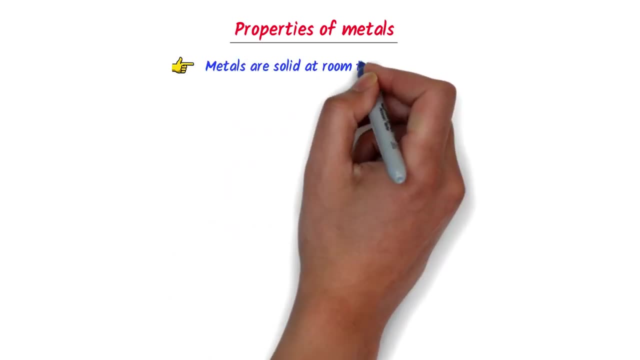 metalloids. all these elements are non-metals. So using this trick, we can easily recognize metals, metalloids and non-metals in the periodic table. Now what are the properties of metals? Well, metals are solid at room temperature, except mercury. Secondly, they have high melting. 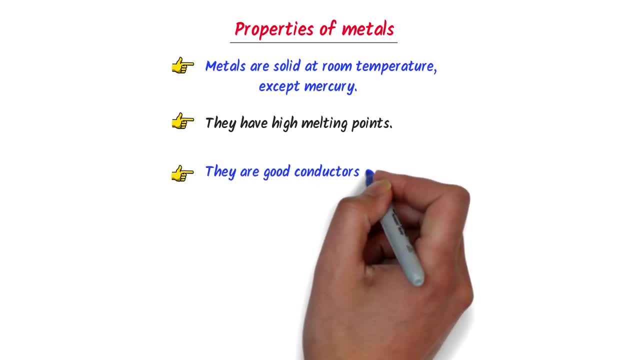 points. Thirdly, they are good conductors of heat and electricity. Fourthly, they are malleable. It means that we can easily bend metals into different shapes. Fifthly, metals are ductile. It means that they can be drawn out into wires, For example. 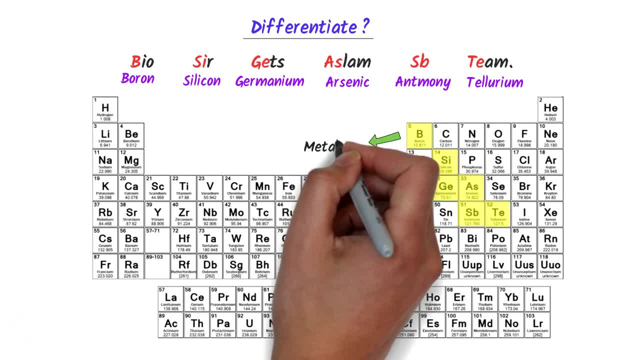 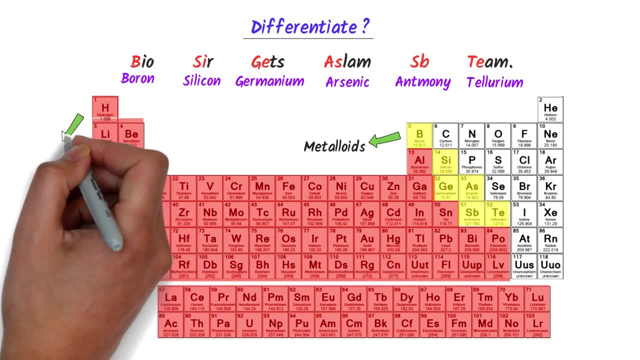 Thus, I highlight all these 6 elements in the periodic table. Now listen carefully. At the left sides of the metalloids, all these elements are metals, While at the right side of the metalloids, all these elements are metals. Now listen carefully At the left sides of the. 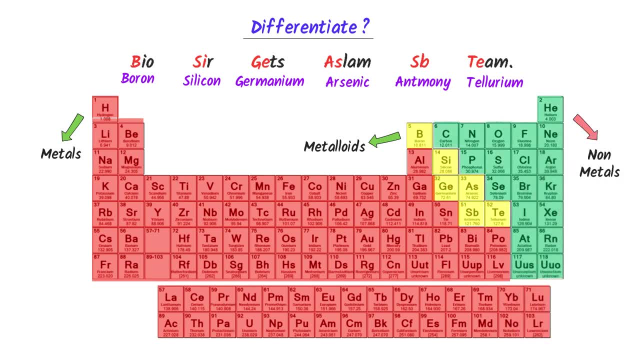 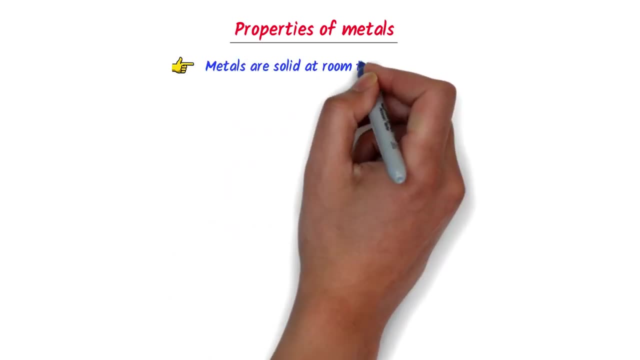 metalloids. all these elements are non-metals. So using this trick, we can easily recognize metals, metalloids and non-metals in the periodic table. Now what are the properties of metals? Well, metals are solid at room temperature, except mercury. Secondly, they have high melting. 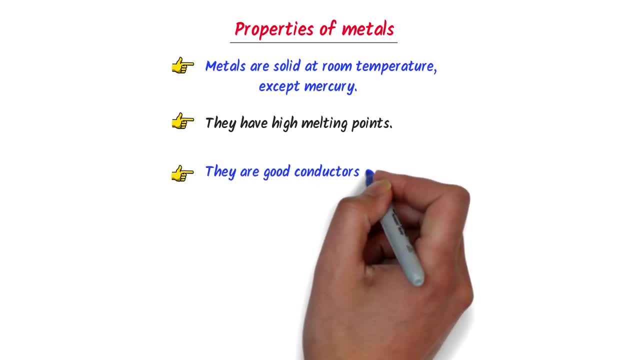 points. Thirdly, they are good conductors of heat and electricity. Fourthly, they are malleable. It means that we can easily bend metals into different shapes. Fifthly, metals are ductile. It means that they can be drawn out into wires, For example. 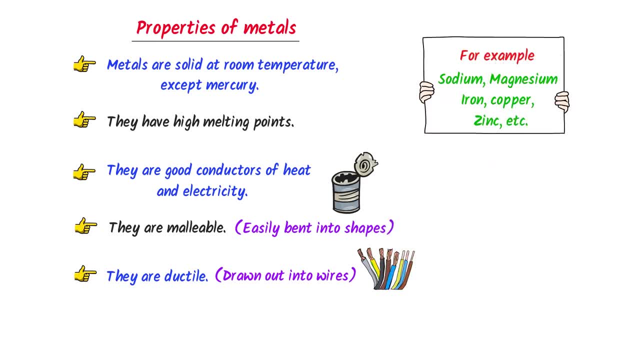 sodium, magnesium, iron, copper, zinc, etc. are all metals. In our daily life, the body of airplane is made up of aluminium And aluminium is made up of aluminium. So in our daily life, the body of airplane is made up of aluminium. So in our daily life, the body of aluminium is made up of. 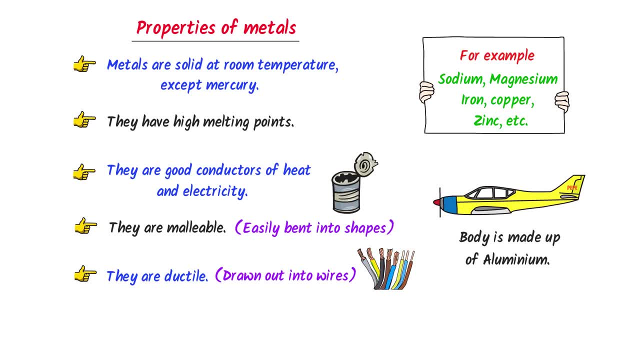 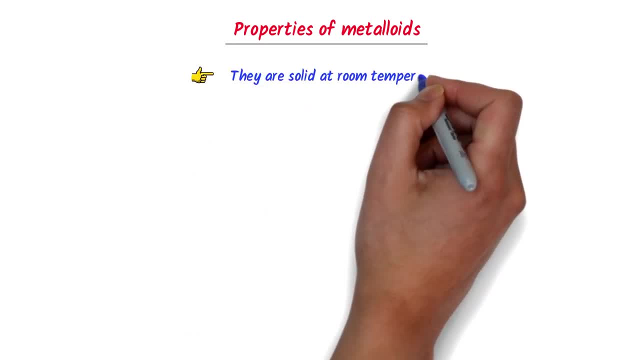 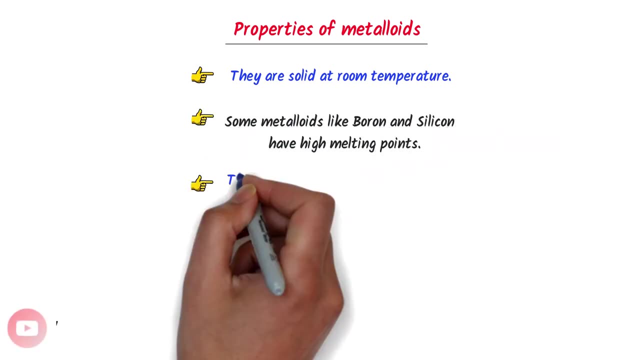 metal. So these are the five common properties of metals. Now what about the properties of metalloids? Well, metalloids are also solid at room temperature. Secondly, they have high melting points. Thirdly, metalloids are semiconductor of heat and electricity. It means that they are not. 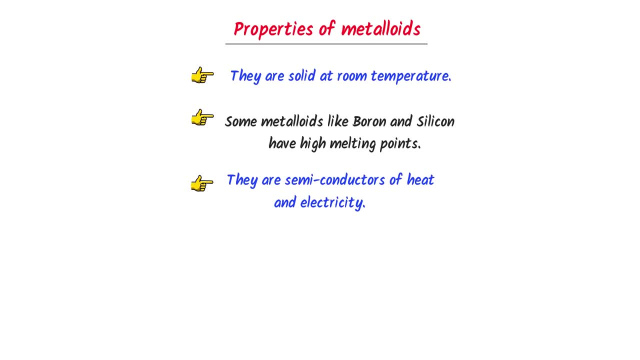 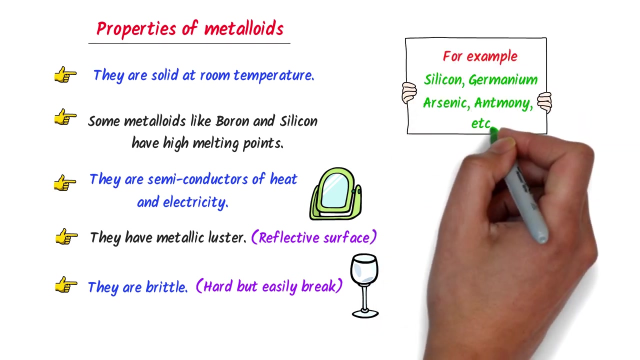 that much good at conducting heat and electricity like metals. Fourthly, they have a metallic luster and generally look like metals. Fifthly, they are brittle. It means that when we apply force to it they are easily shattered. For example, silicon, germanium, arsenic etc are all metalloids.